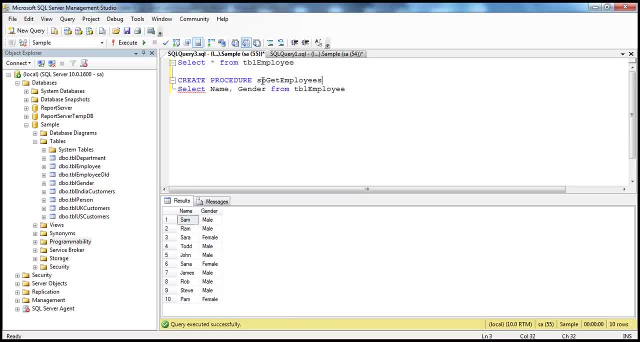 And look at this. in the name I have this letters sp. A common naming convention for stored procedures is that we usually prefix that with small letter s And small letter p, indicating that just by looking at this name you can tell this is a stored procedure. 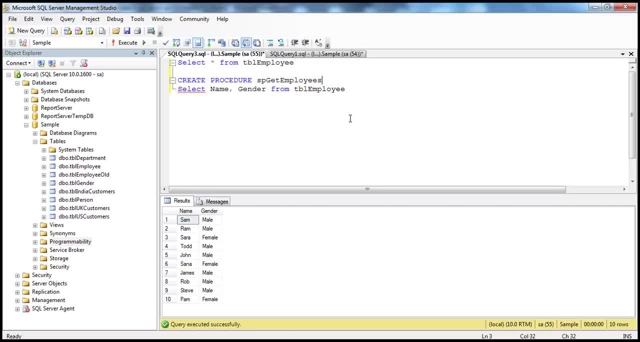 So create procedure, procedure name and then you will use as begin and end. So the definition of your stored procedure goes between this begin and end. So this is the body of your stored procedure. Now, when I execute this command, I'm going to use this as the body of the stored procedure. 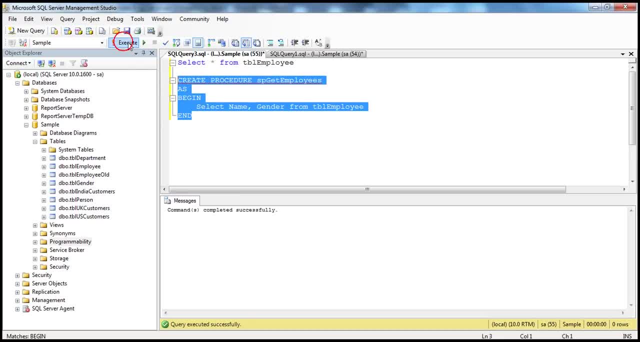 Now, when I execute this command, I'm going to use this as the body of the stored procedure. What's going to happen is a stored procedure with this name gets created in this database, which is構 nothing but sample that we have selected here. 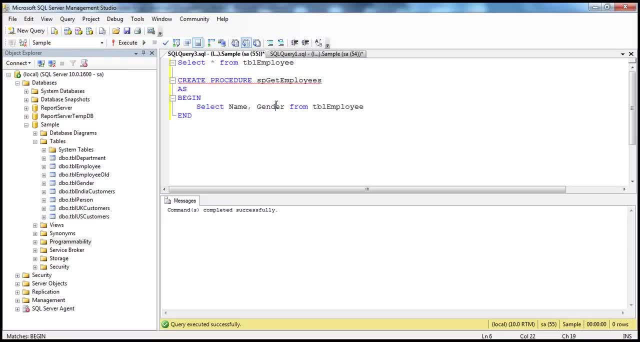 Now, if you want to look at the stored procedure that you have just created, or if you want to make sure if this procedure is actually created or not, go into that database, which is sample, and then you have this folder call programmability- expand that. 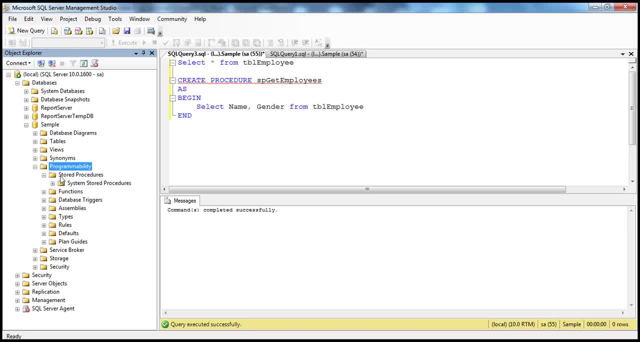 and you should see a folder called stored procedures. If you expand that- you know we don't have it currently listed there- just refresh that and you should see that stored procedure which we have just created, which is SP: get employees. okay, so anytime you want the name and gender of an employee. 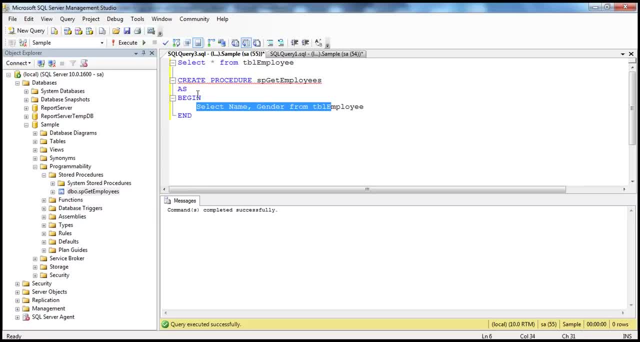 instead of writing this query again, what you can actually do is execute the stored procedure. okay, so if you want to execute, you just need the name of the procedure. so what happens when I execute the stored procedure? okay, to execute the stored procedure. you just highlight that and click execute. 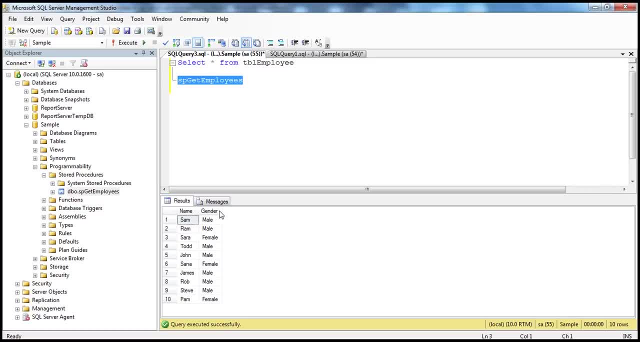 and you get the name and gender. you don't have to write that query anymore. now you might be wondering. it's a very simple query. why don't I write that rather than having to create this procedure and then invoke it? now? this procedure may be simple. in reality, the procedures will be long. 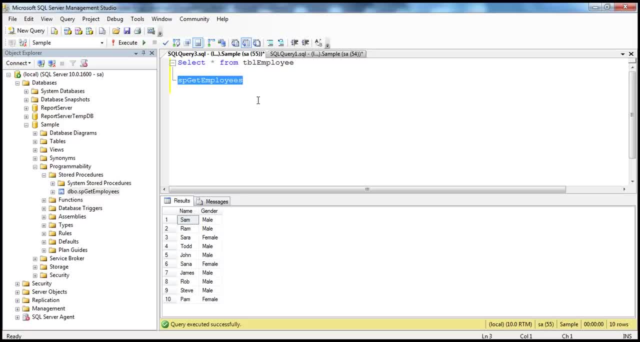 you know that there are very- you know- stored procedures with over three thousands of lines, for example. okay, and not only that, there are several other benefits of using stored procedures, from security to network, reducing network traffic, etc. we will be talking about the advantages of stored procedures in a very great 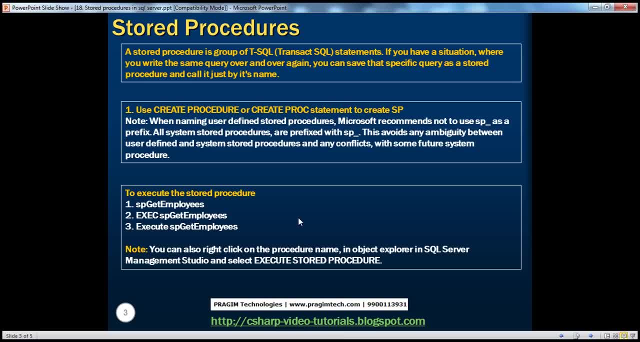 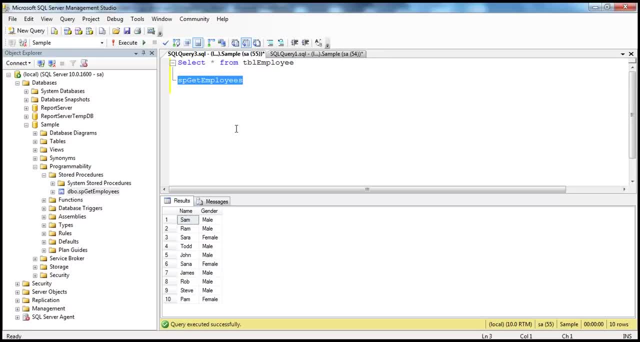 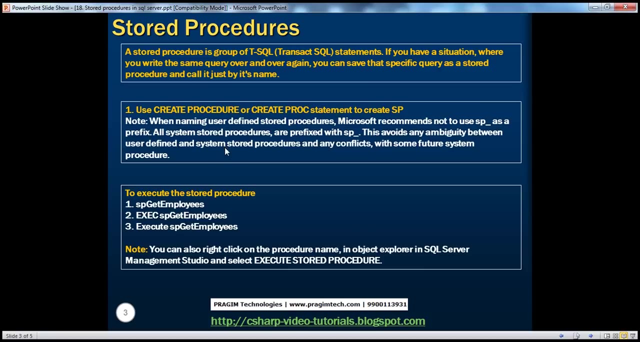 detail in a later session. okay, so we use create procedure or create proc statement to create SP. I mean you can either say create procedure or you can just say create proc for shortcut. okay, to create a stored procedure- we'll talk about the naming convention of the stored procedures in just a bit- okay, and to execute the stored procedure, we. 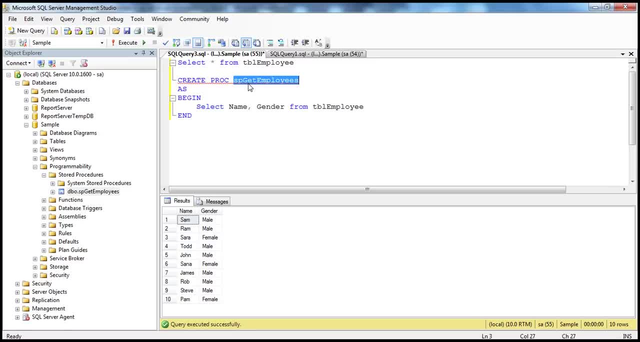 have seen how to execute that stored procedure. you know, you just copy that- the name of the stored procedure- and you click this execute button and what happens? the SQL statement within that stored procedure gets executed and it returns the name and gender columns. alright, so that's where one way to 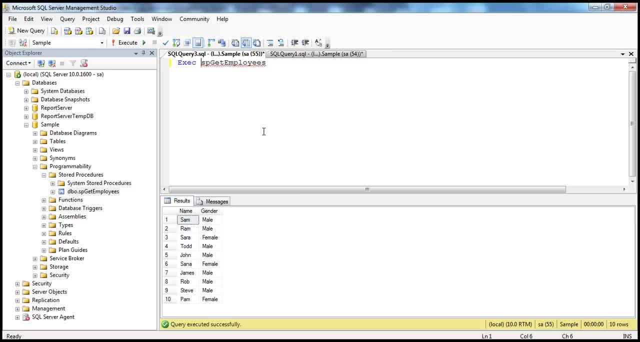 execute it, or you can use the exec keyword and then click this, or you can you can use a full execute keyword and then again press F5, or you can also graphically execute the stored procedure: just right click on the stored procedure and select execute stored procedure. 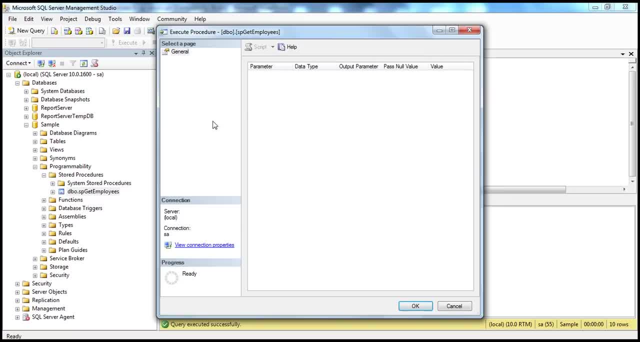 and the moment you do that, it shows this window. this procedure doesn't have any parameters. otherwise you'll have to supply the values for the parameters. in just a bit we'll see how to create a stored procedure that takes parameters. now, when I click OK, it executes that stored procedure. 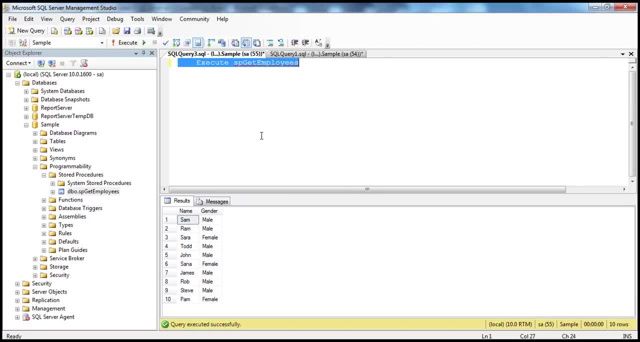 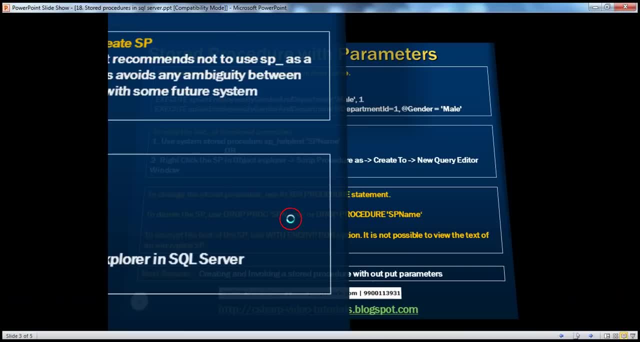 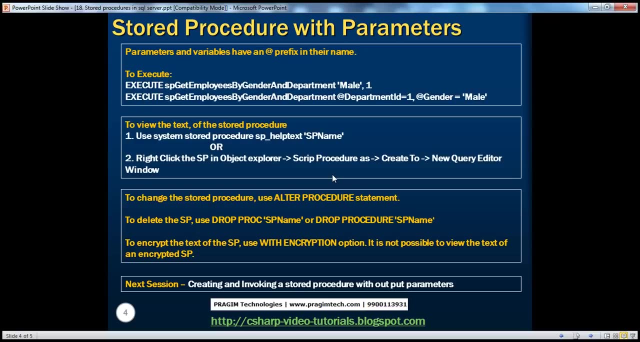 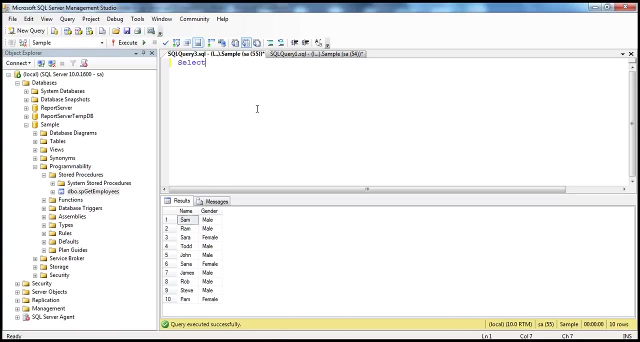 look at that. all right, so those are the different ways to execute stored procedure. now let us look at a simple example of how to create a stored procedure with parameters. ok, so let's go back to that table: tbl employees. all right, now what I want to do is 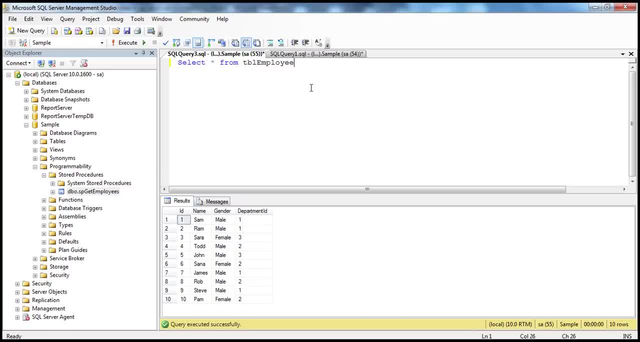 I want to create a stored procedure which takes two parameters, maybe gender and the Department ID. ok, for example, if i pass gender as male and department ID as one to your stored procedure, it should give me employees only within that gender and within that department. ok, so your stored procedure needs to have these parameters. 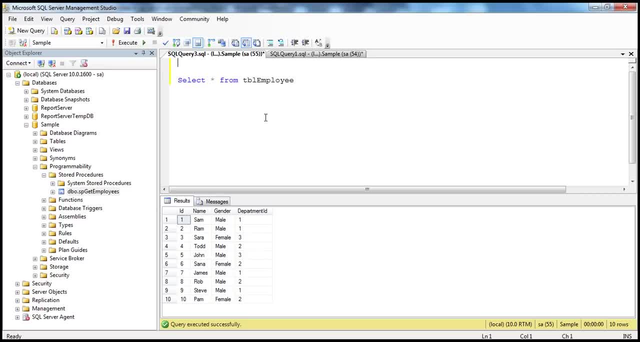 ok, so let's see how to do that. so, as usual, to create a stored procedure, we use create procedure command command. so create procedure and give your procedure a meaningful name. so sp: get employees by gender and department. okay, so i want the employees by gender and department now look at: 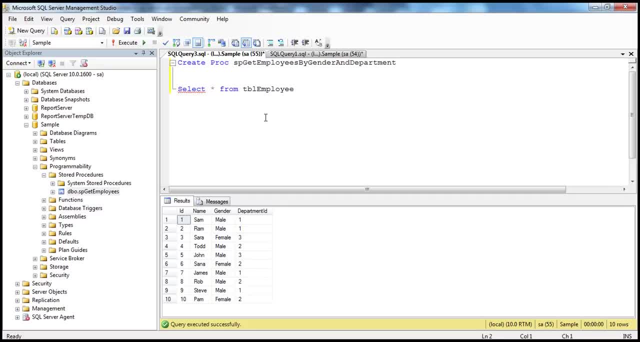 this now, this procedure: okay, the user who invokes your stored procedure is going to pass the stored procedure, the gender and the department id. so for them to be able to pass the values for gender and department id, they should be parameters, just like how functions have parameters in c, sharp or any. 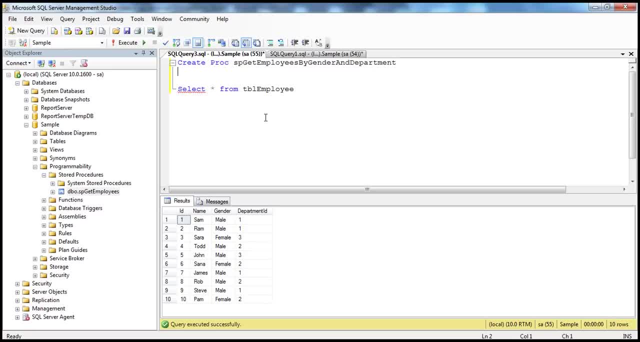 other programming language. stored procedures can also have parameters, okay, so one is the gender parameter and if you look at gender, it's text here. so the data type is going to be n, where care of maybe 20, and department id. department id is going to be integer, so department id integer as begin, and so the definition of your. 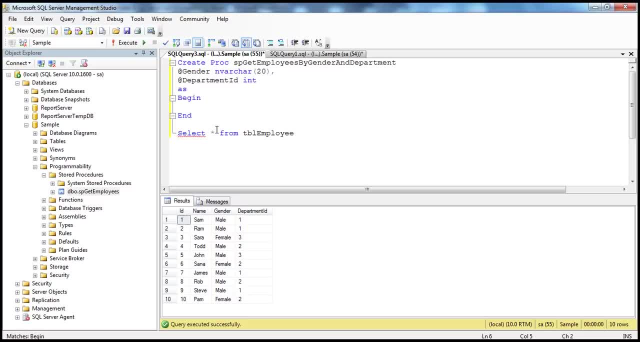 stored procedure goes in between these lines. okay, so what do we want from the table? we want the name and maybe just the gender and also the department id. from which table? we want it from tbl employee table. but we don't want all names, genders and department ids. we want to filter them with what the user is. 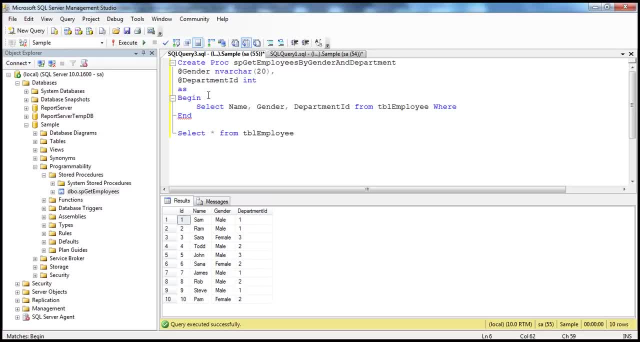 going to pass in is going to pass in the gender and department id. so we are going to say the gender column here should be equal to whatever the user is passing in at gender and along the same lines and department id- let's bring this to another line- is equal to whatever the 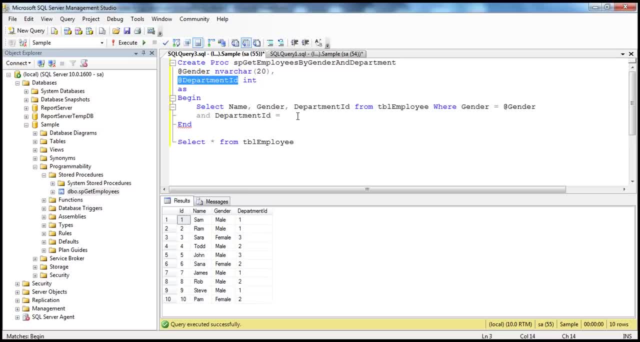 user is going to pass in. okay, so these parameters are like placeholders. when users execute your stored procedure, they're going to pass in values for this gender and department id, which will be replaced at execution time. okay, so let's create this store procedure so to create that, select the entire. 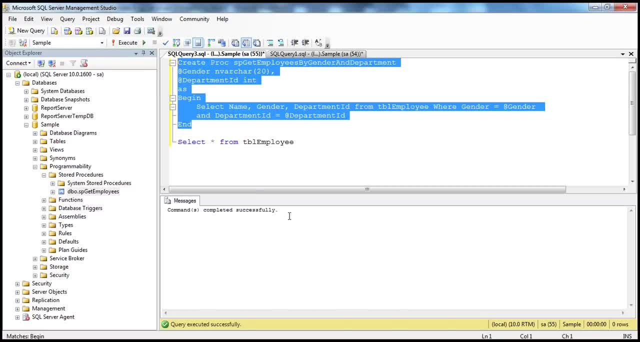 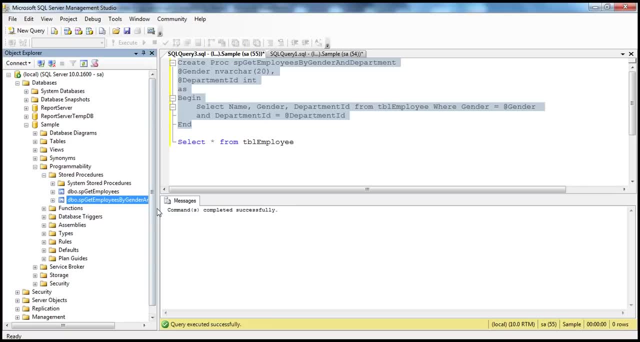 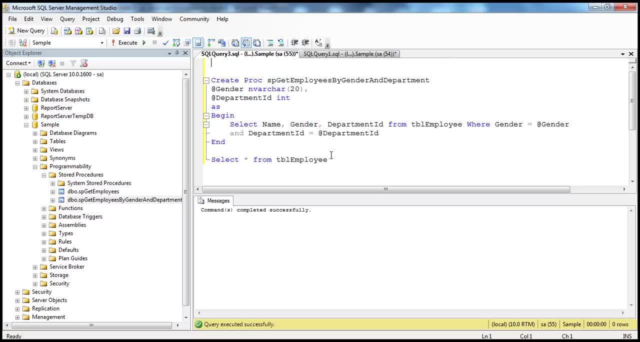 store procedure: click execute button command completed successfully. now if you refresh the stored procedures folder, you should see SP get employees by gender and department. okay, now to execute this stored procedure. i just need the name of the stored procedure and look at this. this stored procedure now is. 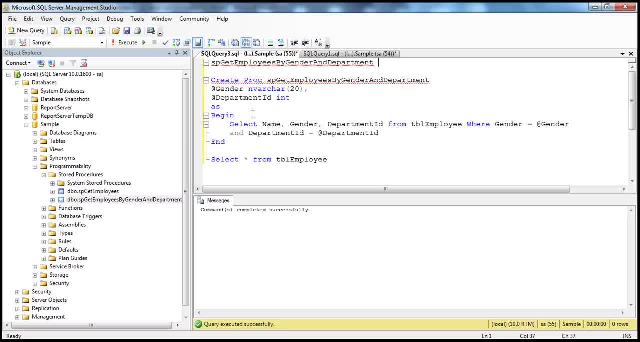 expecting gender and department id parameters. now look at this: if i don't pass the parameters and if i just try to execute that stored procedure- see highlight that- and then press execute- what's going to happen? this procedure or function sp get employees by gender and department. expects parameter at gender, which was not supplied, and that makes sense. it's expecting 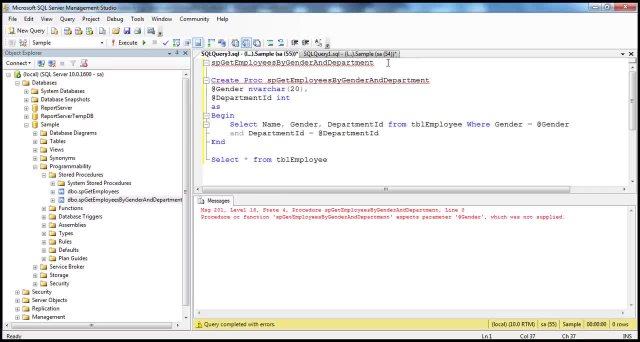 a gender parameter which is not supplied, so we need to pass in the gender parameter, since gender is of type n, where car i have to use single quotes. so i want the male employees within you know department id one, so department id is one. so these are the two parameters that 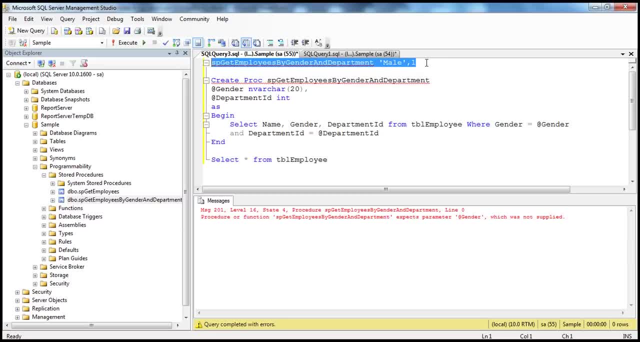 this two the stored procedure expects and we need to pass them. so when i press f5- now look at that- i only get male employees within that. you know department id one. okay. on the other hand, if i want all the male employees in department id two, i can do so. 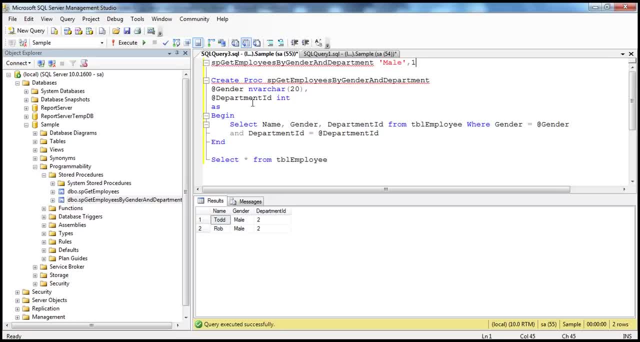 all, right now, when you have parameters like this, you know what you're doing is you're just passing in the parameters, so so. so this male value will be taken into at gender parameter, whereas this number one is passed into department id parameter. okay, now what happens if i put it the other way around? i am passing one first, okay, so what's? 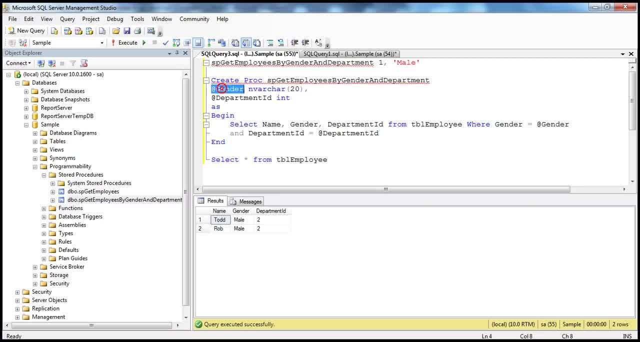 going to happen. it will take this one into gender and one is an integer, but gender is of type n where car and this one will be converted into n where car, implicitly, no problem. but it comes to the second parameter, male it. it tries to take this into department id parameter and if you look at the data type, 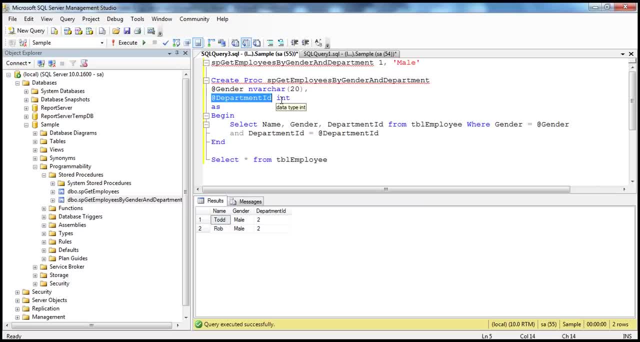 of department id parameter. it is integer, okay. so it tries to convert this string into integer and it fails and it throws an exception. look at this: if i try to execute this now, i get an exception saying that error converting data type where car to integer. so it is trying. 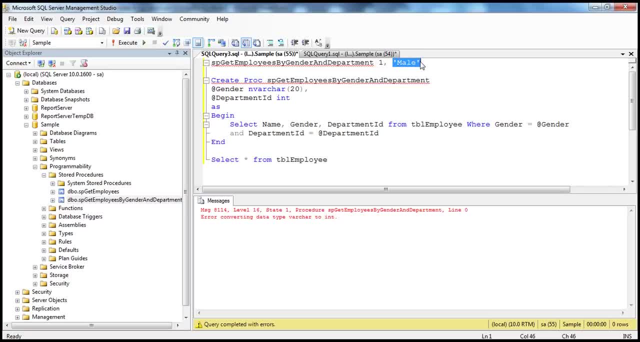 to convert this male, you know, string of type n, where car, into integer and we get that error. okay, so when you have multiple parameters, that is true. procedure is expecting. and if you're passing just values, the values order, you know, the order in which you pass them is important. okay, the first parameter will: 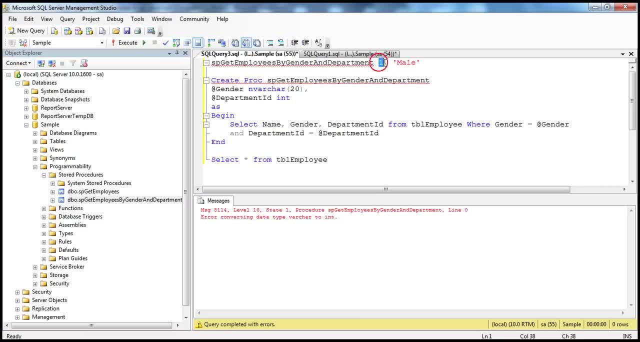 be used- i mean the value here- the first argument will be used with the first parameter and the second argument will be used with the second parameter. okay, that's why the order is important. but if you use the parameter names like this- let's say, i want to pass one to at department id- i can specify the name of the parameter like: 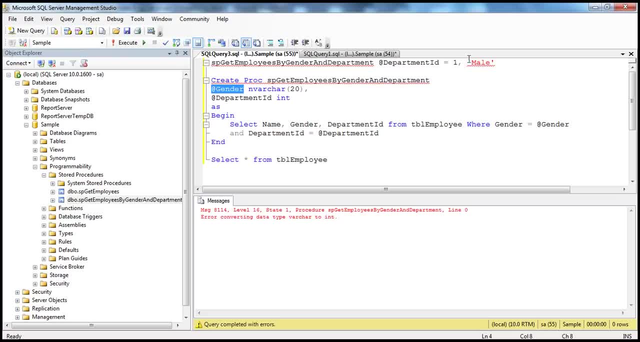 so, and similarly, i can specify the name of the parameter for gender. so when i execute this now, i will have no issues, because you are specifying the name of the parameter. okay, so sql server knows. okay, this one is, and you know to be, the value for department id parameter and male is the value for gender. 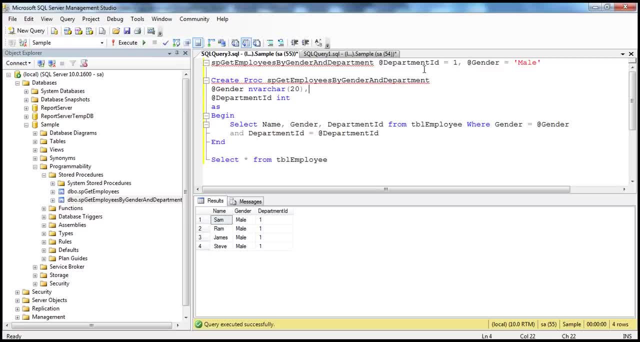 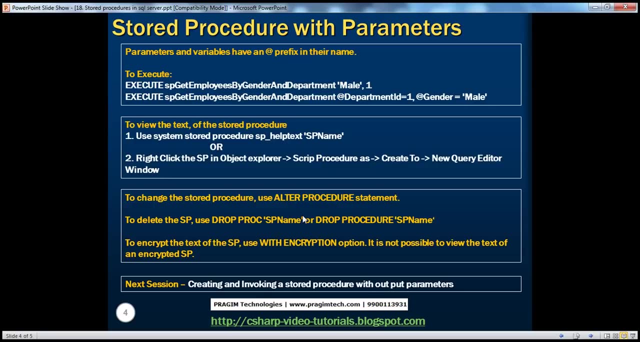 parameter. it's only when you don't specify the names of the parameter. the order of the- the order in which you pass the parameter, is parameters- is important. all right and okay. so we have seen how to create a simple stored procedure and how to create a procedure. 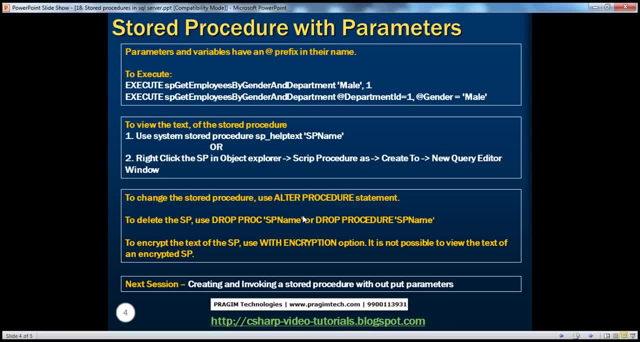 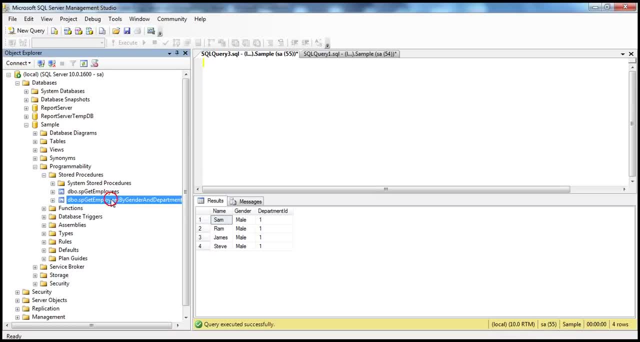 with parameters as well, and we have seen how to execute them as well. okay, now, once you have written the stored procedures, let's say i have created two procedures until now: spget employees and spgetemploys by gender and department. now, if i want to view the text of these stored 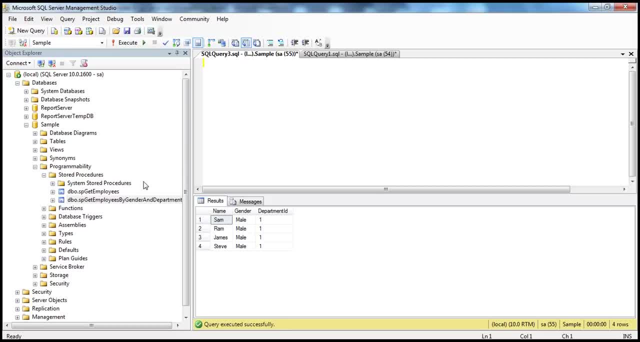 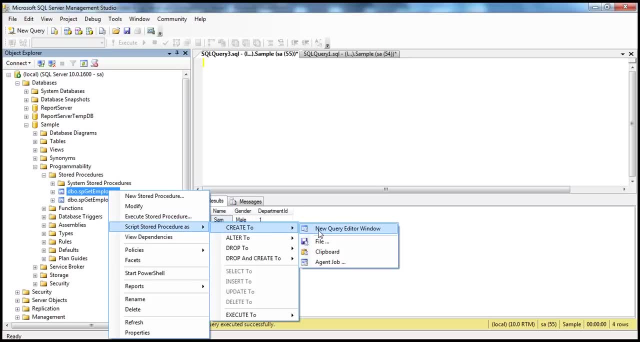 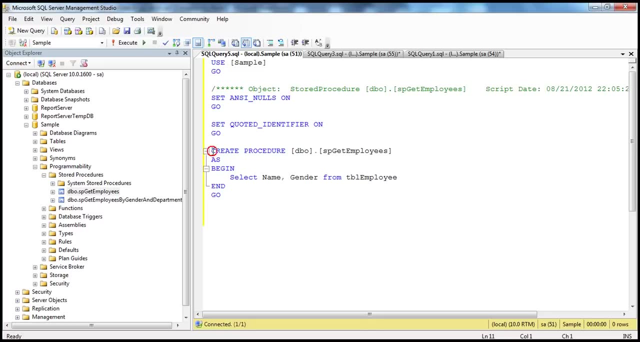 procedures. what are the different ways that are available? one way is to simply right click on that stored procedure script- stored procedure as create to new query editor window. this, you know, generates the contents of that stored procedure. look at this. this is the stored procedure definition that we have created. 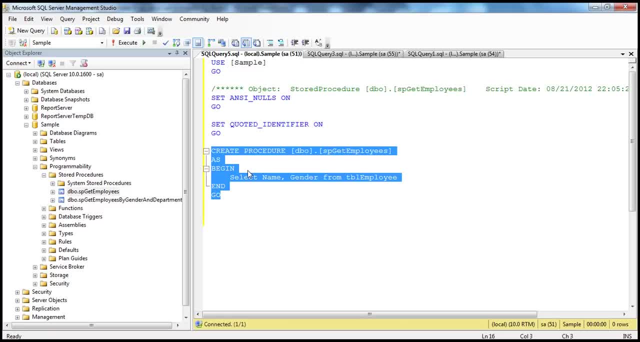 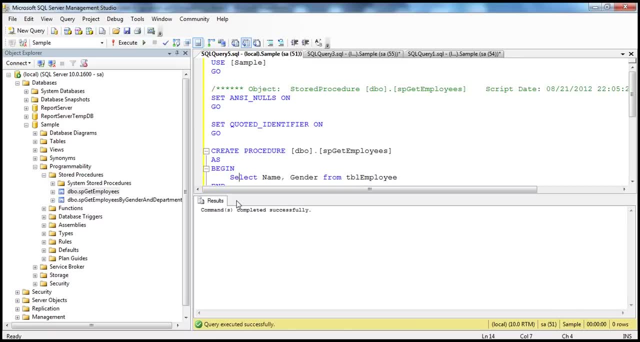 Create procedure, procedure, procedure name as begin, end and then our query. This is one way to look at the definition of a stored procedure and the other way is to use a system stored procedure. You know, these stored procedures that we have created here are user defined stored procedures. These are not system. 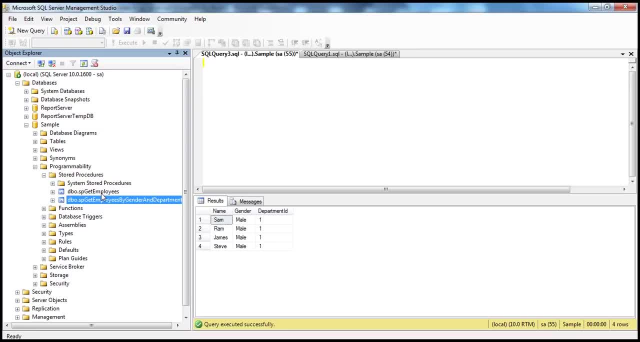 stored procedures. Now, SQL server, you know, has some system stored procedures defined, okay, and we use it for certain tasks. For example, I want to find the text of a stored procedure. How do I do that? I can use a system stored procedure called SP underscore help text, okay. So look at this This: 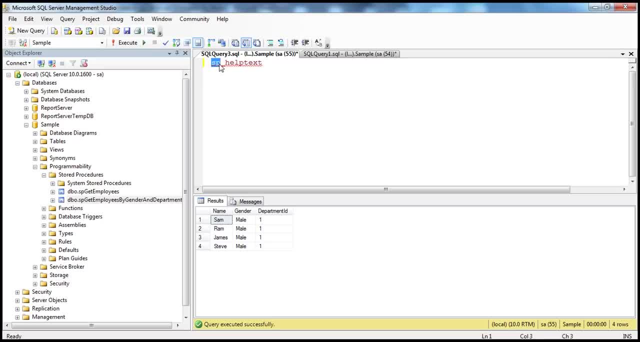 is the name of the system. stored procedure: SP. underscore: help text: okay, SP, help text. and then if I pass in the name of the stored procedure there, SP get employees and then when I select this, I can use it for certain tasks. So I can use it for certain tasks. So I can use it for certain. 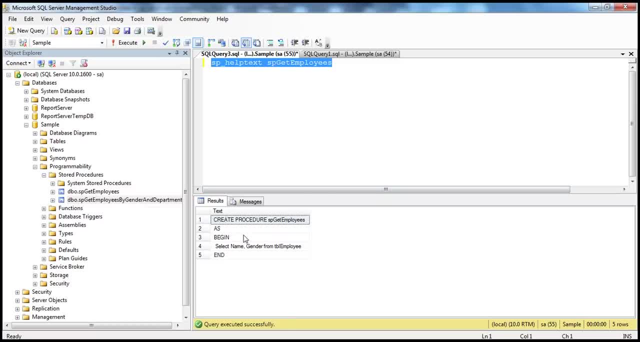 tasks. Let me pick them together and execute this. Look at this. I get the text of my stores here. You can then copy that, paste it here and see how does the implementation of the stored procedure looks like. okay, So to view the definition of a stored procedure, you can either right click on: 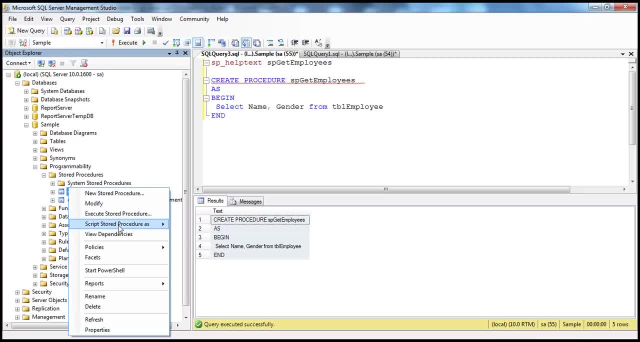 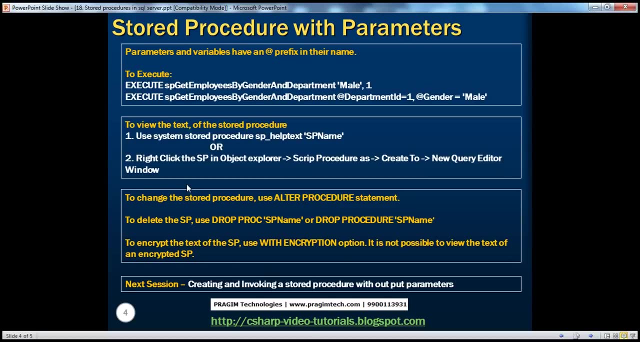 that Script stored procedureS- create to new queryaditorWendow or you can use the system stored procedure SP underscore help text followed by the name of the stored procedure. but it is, which gives you the text of the stored procedure. okay, now in this slide, if you look at this, you know. 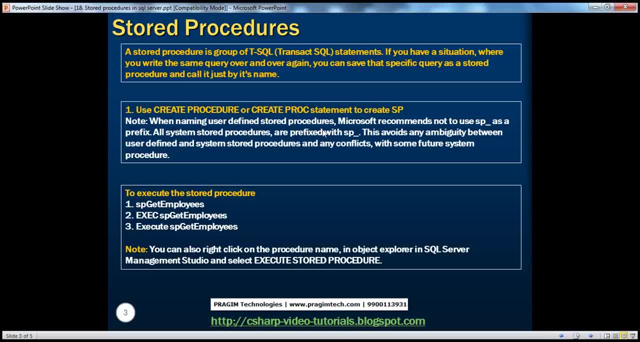 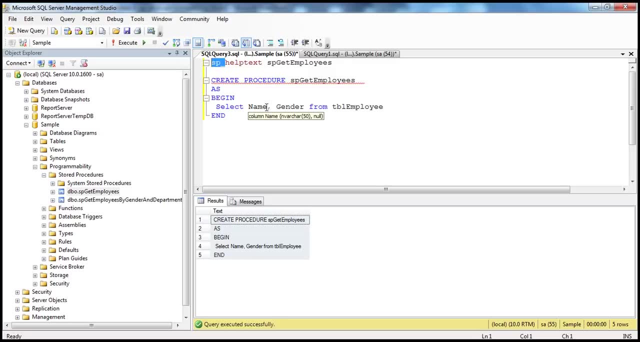 whenever we name user-defined stored procedure, Microsoft recommends not to use SP underscore- you know prefix for user-defined stored procedures- because the reason is: system stored procedures has that prefix. okay, now, if you happen to use SP underscore prefix for your user-defined stored procedures, there are two problems. 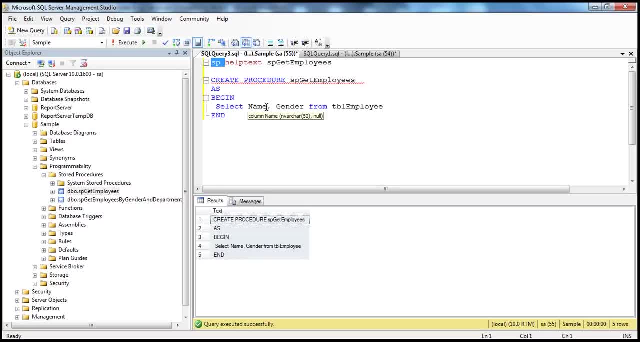 number one: there will be an ambiguity between user-defined stored procedures and system defined stored procedures. just by looking at the name, we cannot tell. you know, is this a user-defined stored procedure or system defined stored procedure? okay, and another problem is with future releases of, you know, new SQL Server version. 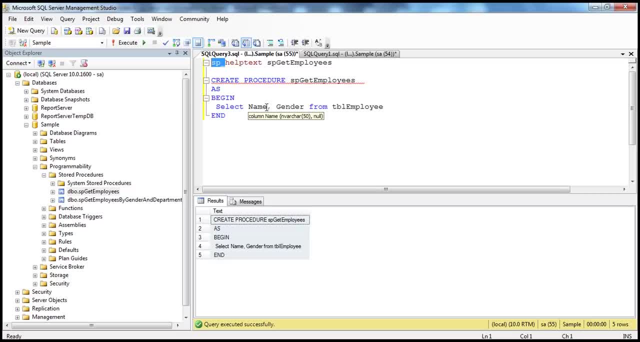 there may be name conflicts. you know, if you create, let's say, SP underscore get date, you know, stored procedure, and in a future release there is a system stored procedure which is, you know, similarly named SP underscore get date, you know it's gonna conflict with the user stored procedure. 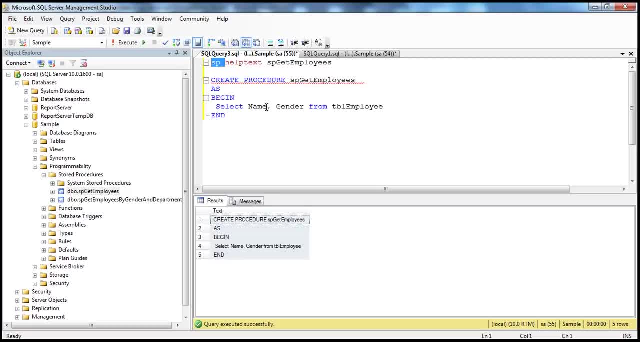 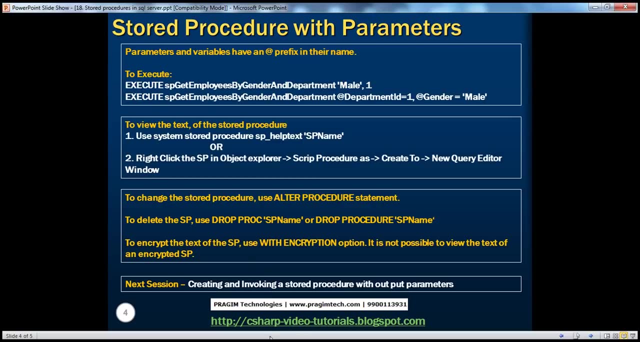 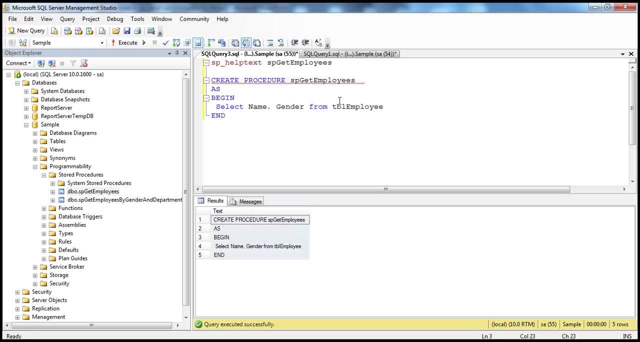 okay. so to avoid problems like this, it's always better not to prefix user-defined stored procedures with SP underscore prefix. alright, so to change the stored procedure. now, once we have created a stored procedure- for example, I have the stored procedure SP get employees. after I have created the stored procedure, let's say I want to change its implementation. 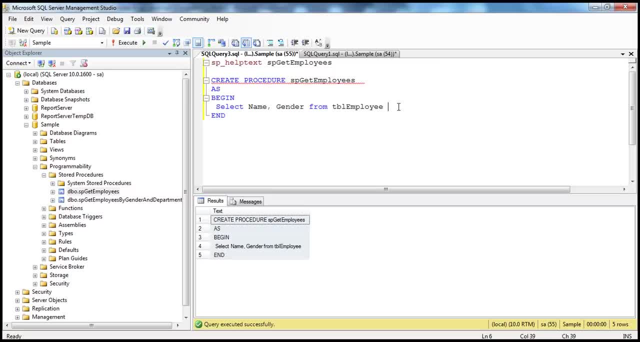 in some way. how do I do that? let's say, at the moment when I execute this SP- get employees stored procedure, I'm not getting the names sorted, you know? I mean the names are basically not sorted. I want them to be sorted, so how do I do that? 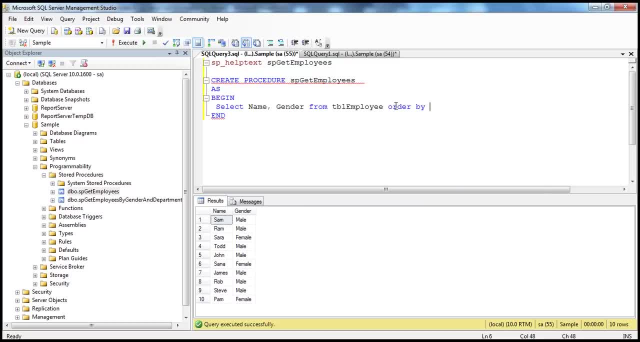 I will use the order by clause, so order by name. okay, so I'm changing the implementation of the stored procedure. now, if I execute this create procedure once again- look at this- we get an error stating that there is already an object named SP- get employees. why we already have that and we are trying to create that again with the same. 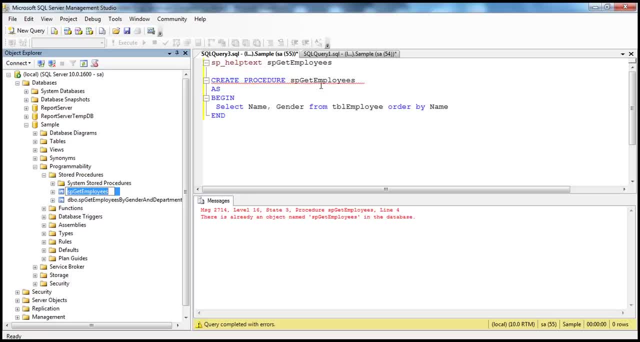 name. so obviously we get that error. our intention here is to change the definition of that stored procedure, not to create another stored procedure. so if you want to change the definition of the stored procedure, then you say alter procedure and I press F5, the stored procedure gets changed. 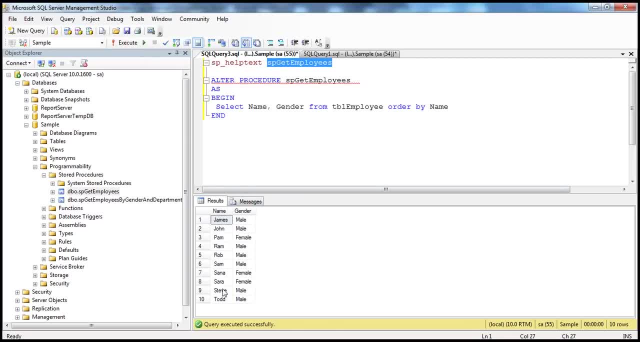 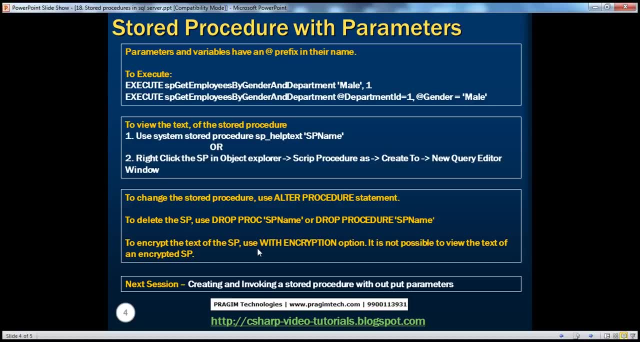 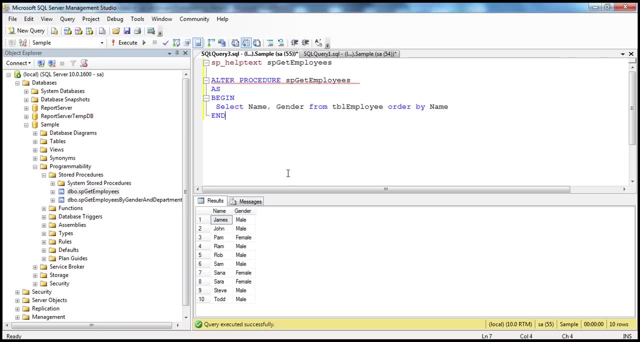 now, if we execute that, we should have the name sorted. okay, so we use alter procedure statement to change the definition of the stored procedure and to delete the stored procedure. we use drop procedure procedure name, just like you know. if you want to drop a table, you will use drop table table name, okay. 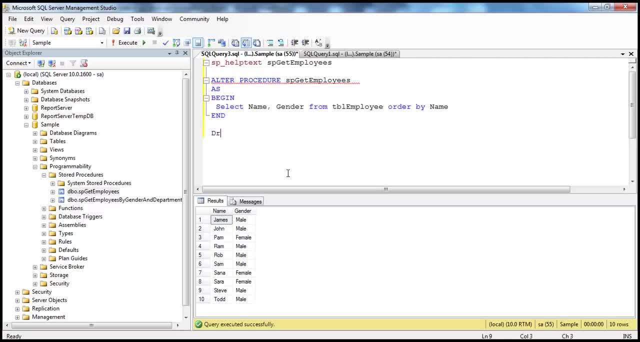 so, similarly, to drop a procedure, you will say drop procedure and procedure name. for example, I want to drop or delete SP, get employees and I just pass it there, I press F5 and then if I refresh the stored procedures folder it's gone. now it's deleted, or what you can do alternatively. 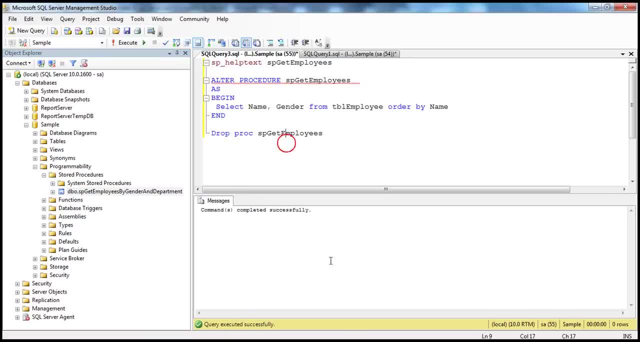 right click on that and select delete. okay, now it's also possible to encrypt the text of the stored procedure, and it's very simple to do. for example, I have this stored procedure now, okay, so as we get employees by gender and department, look at this now. this is not. 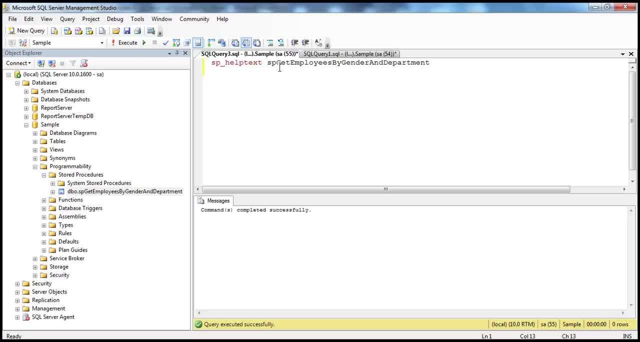 encrypted at the moment. so when I use SP underscore help text and when I press f5, I am able to get the text of that stored procedure. so that's how the stored procedure is implemented. now, if I want to encrypt the contents, the text of the stored procedure, I can do that. how do I do that? all you have to do is to use 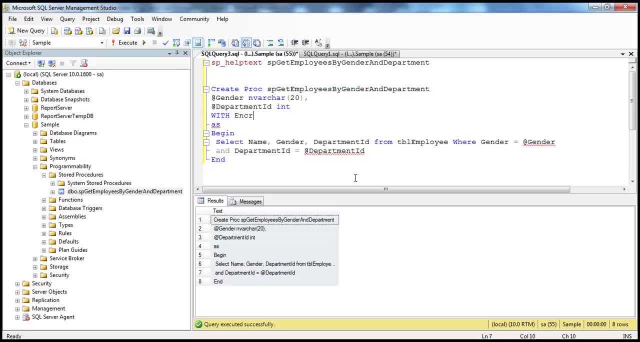 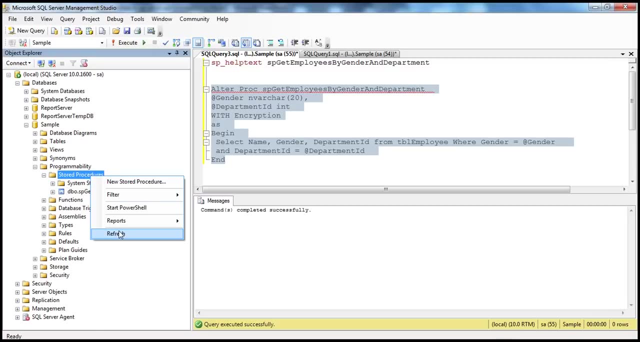 this, switch, this option with encryption- okay, and we want to alter that, so I will say alter. now, when I press f5, look at this, command completed successfully. and now, the moment I refresh this folder, look at this. we get a little lock symbol there indicating that this stored procedure is now encrypted. okay, now, if 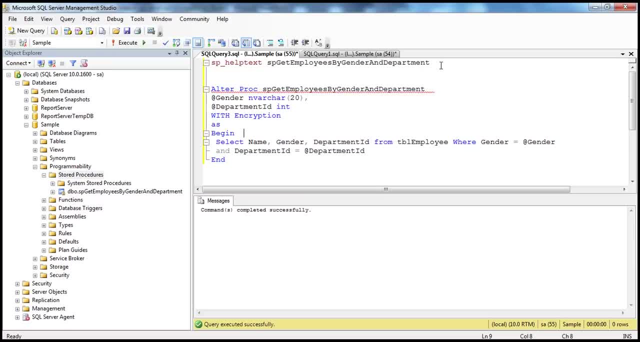 somebody is using this procedure and they want to use this procedure. they already tries to, you know, get the text of the encrypted stored procedure. we get a message saying that the text for the object is encrypted and and we cannot retrieve the text of that. okay, and you get the same kind of message when you 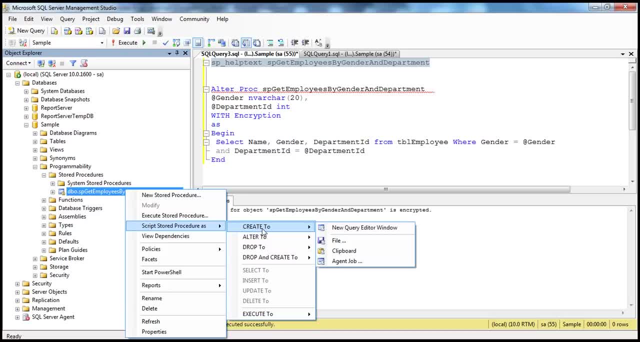 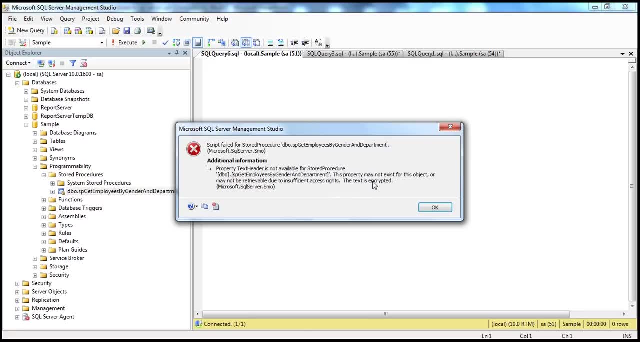 kind of use script stored procedure as create to new query editor window. okay, we get this error box, you know. if you look at here it says the text is encrypted. so once a stored procedure is done and the stored procedure is encrypted, you cannot view the text of that stored. 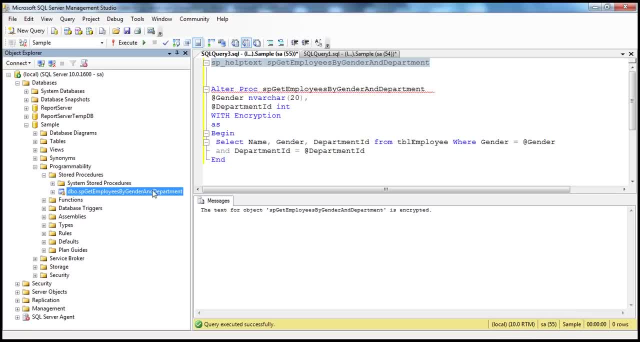 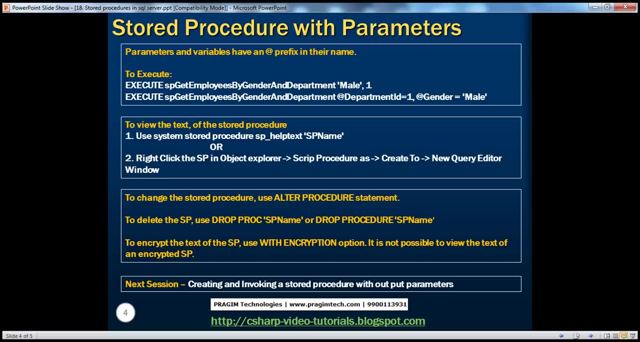 procedure. but, however, if you want to delete the stored procedure, you can go ahead and delete it and now just right-click and select delete, it gets deleted, but you cannot view the contents of a stored procedure. that is encrypted. all right, in the next session we will see how to create and invoke a stored. 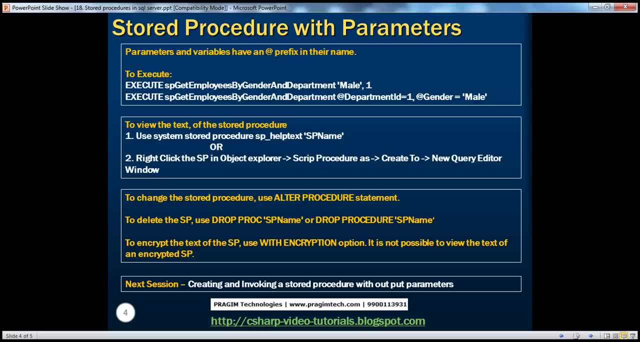 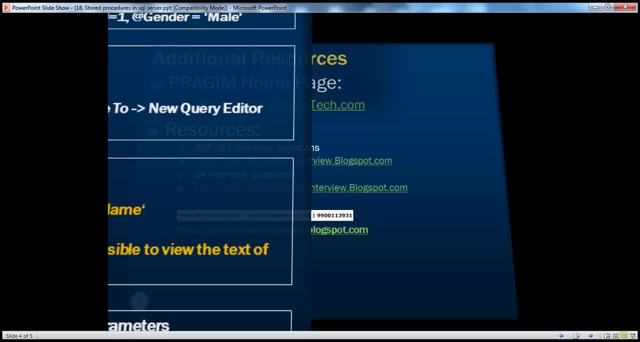 procedure with output parameters. in this session, we have seen how to create a stored procedure with input parameters. in the next session, we'll talk about creating stored procedures with output parameters. on this slide you can find resources for ASPNET and C sharp interview questions. that's it for today.